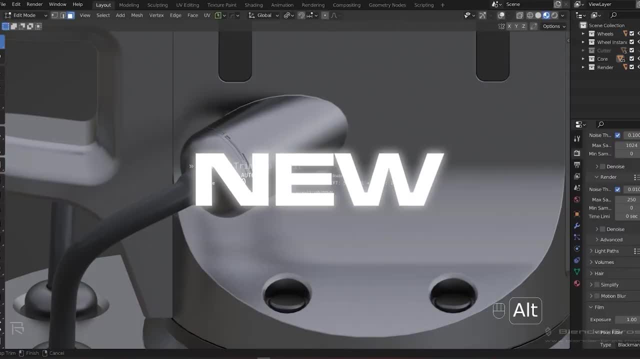 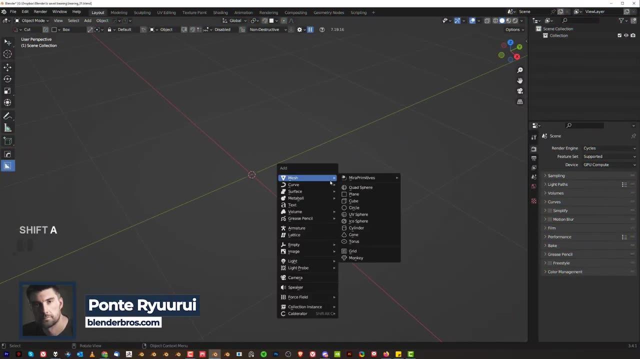 modeling, but also confident with rendering and excited about your new game changing portfolio. Link is in the video description. Let's get started, Alright. so we're gonna start with a cylinder- Shift-I-N cylinder- right- And we're gonna go here and increase the number of segments to 80.. 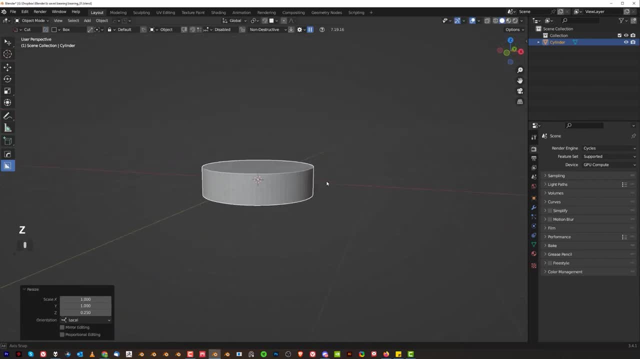 S, Z and scale it down, and I think this is good. Now we're gonna flip this on X so I can work on from the front. I like to work like that, Okay, so let's just sharpen this and let's go. 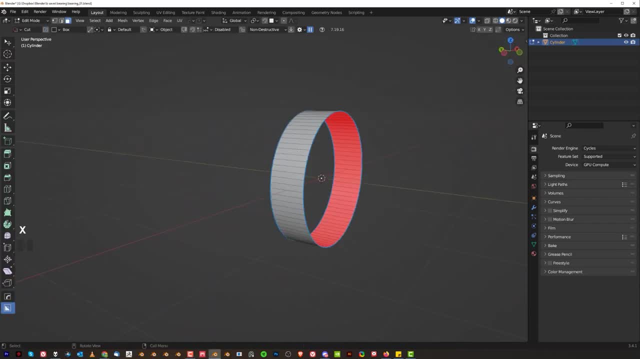 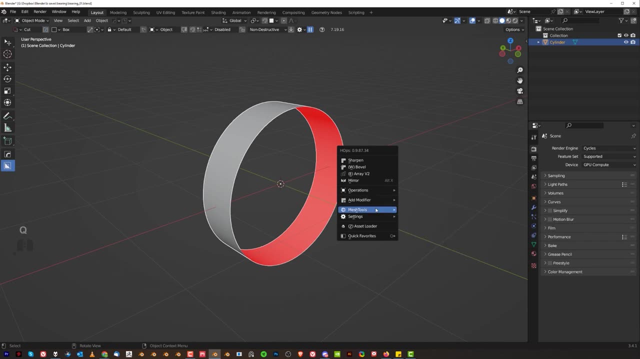 So first of all we're gonna do is we're going to grab these and delete them And we're gonna solidify This middle part. okay, So Q, and we're gonna go to modifiers and solidify, And this will do, And then we also need another one in the middle. 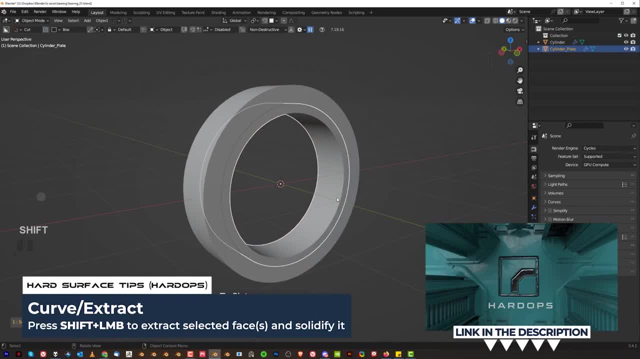 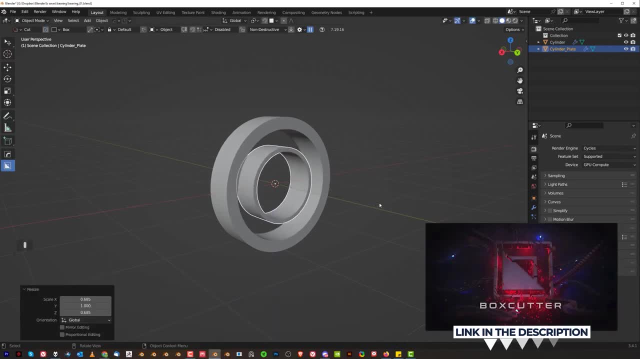 So select that and Q and shift-Curve-Extract and move it inside. I'm gonna scale it down so S and shift-Y, so it scales on X and Z. I go down here like this and it's cool, Let's make it a bit thicker. 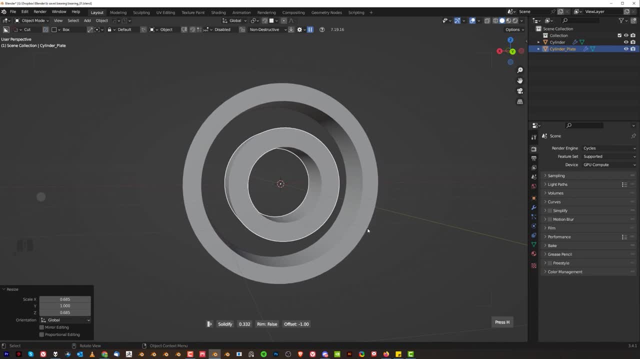 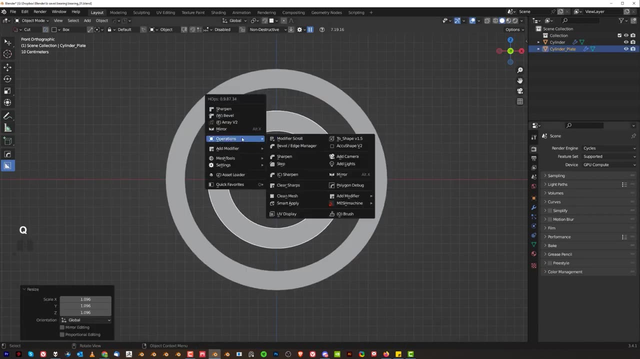 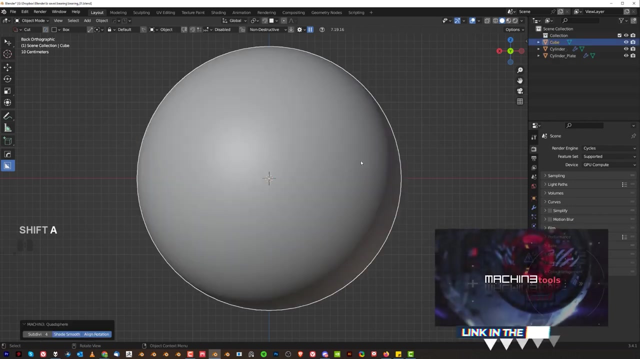 So thicker, Kind of like that. That will do Cool. So now what we need is some bearings. It's actually a bit too fat, you know. Hang on, That's better. So here we're gonna add a quad sphere with machine tools and G-Z. 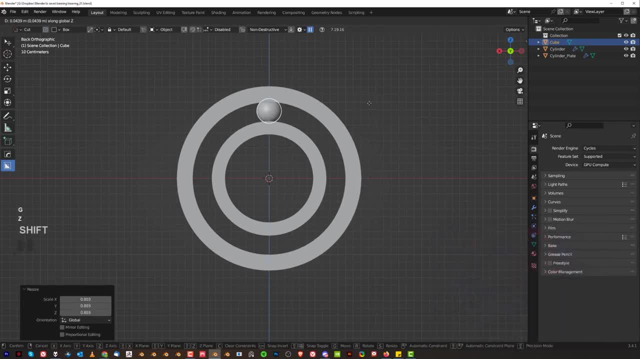 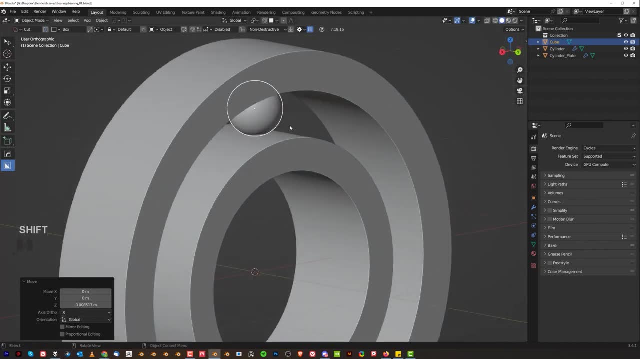 Move it in here, Scale it a bit Now. this ball needs to, you know, needs to be touching both sides, And we're gonna create some, some grooves here so it can be a little bit larger than this casing, Okay. 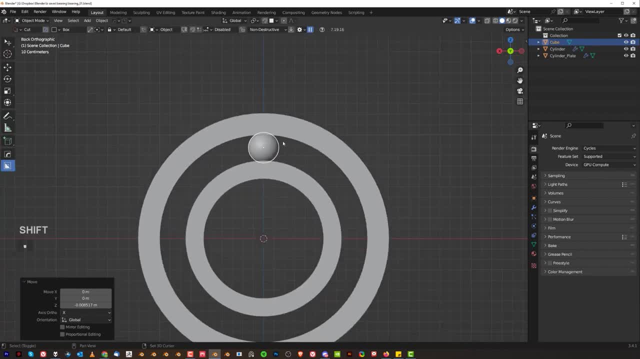 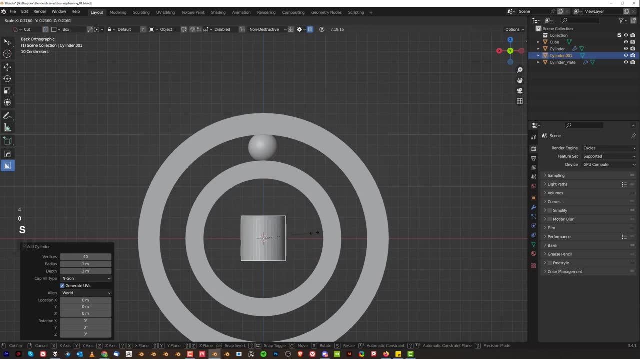 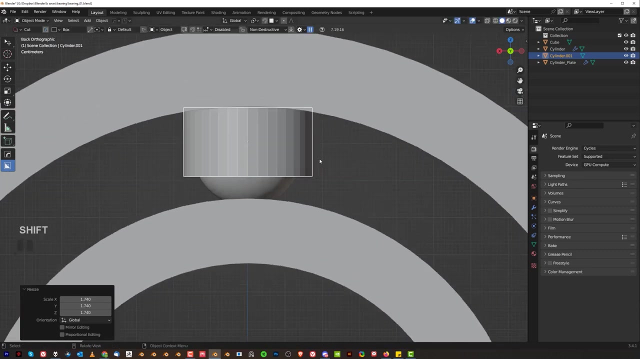 And we're going to add sort of like a casing on top of it. So another cylinder And we're gonna change it to maybe 40 and scale it down and bring it up And squash it down and scale this And we need to fit it in here. 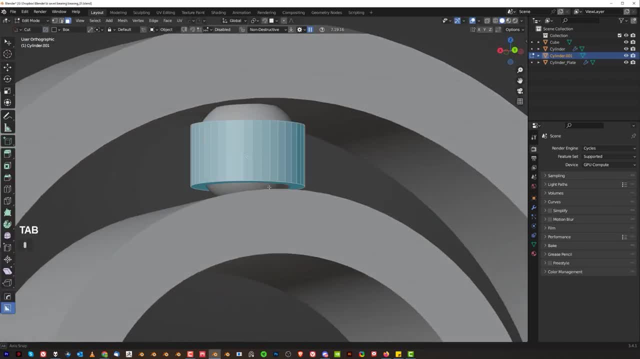 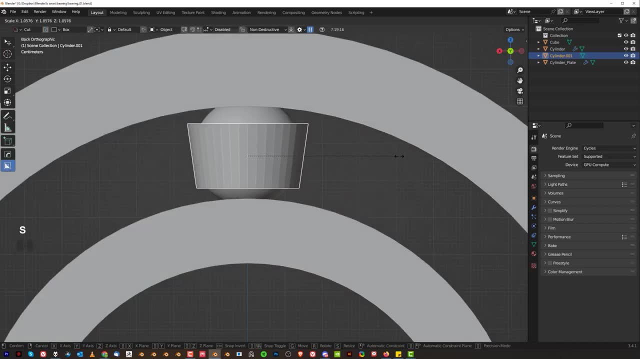 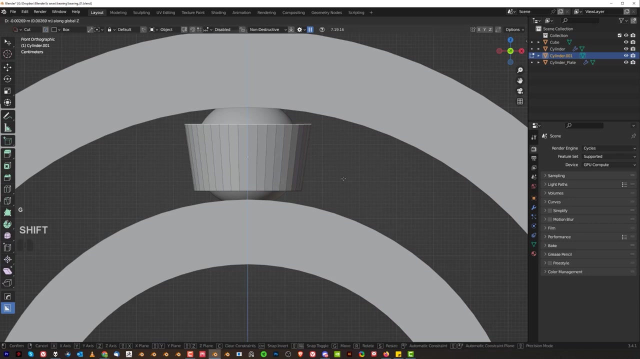 So a bit smaller, And we're going to scale it in there here like this and then make it a little bit fatter. there we go, maybe not as tall, yeah, so jay-z. and there we go, maybe not as not as low here. so, jay-z, i think that will do, maybe a little. 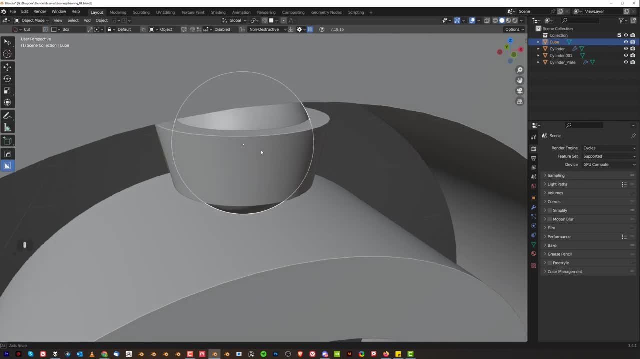 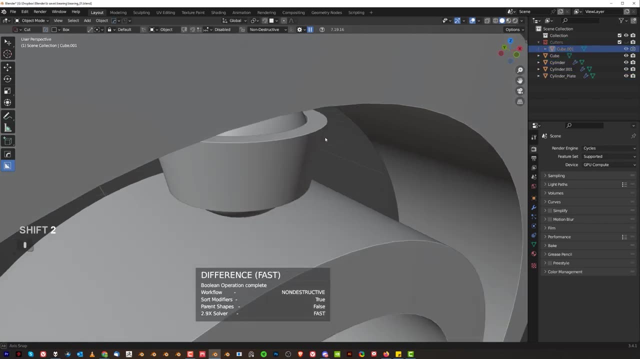 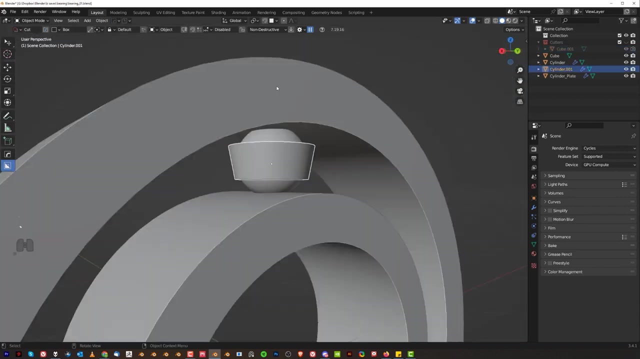 bit bigger. there we go and sharpen- cool, we could technically cut it out, um, if you want to. so shift the skeletal a little bit, and you know difference. uh, so you're gonna get this kind of a- you know precise sort of a cut out, and which is fine and i think we're good to go. so let's apply scale here. 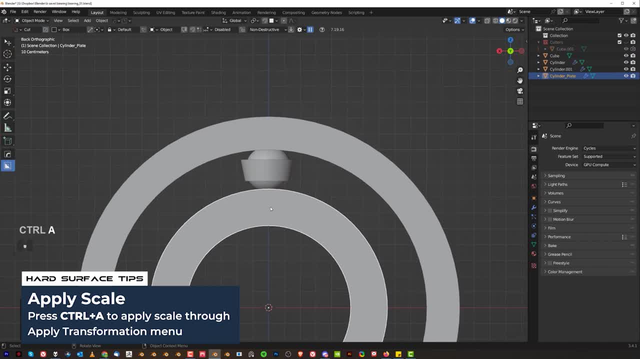 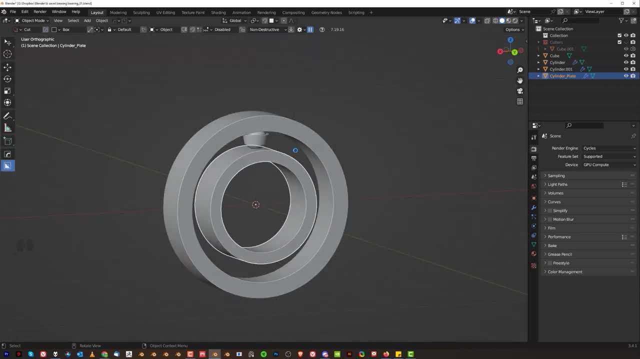 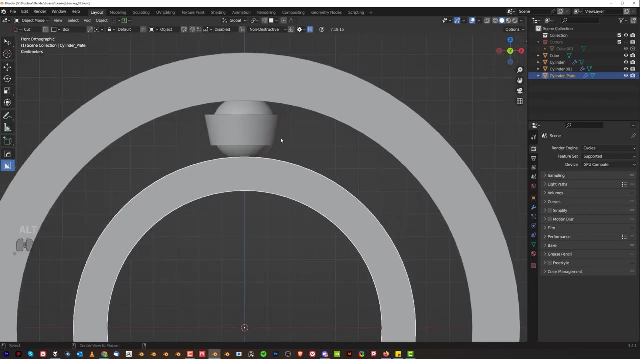 apply scale here. apply scale here and apply scale here. okay, and let's just fix this solidification. when you apply scale and solidification after resizing you might see some- you know- size shift, so let's fix it. okay now. cool. so here here, what we're gonna do is we're gonna select that. 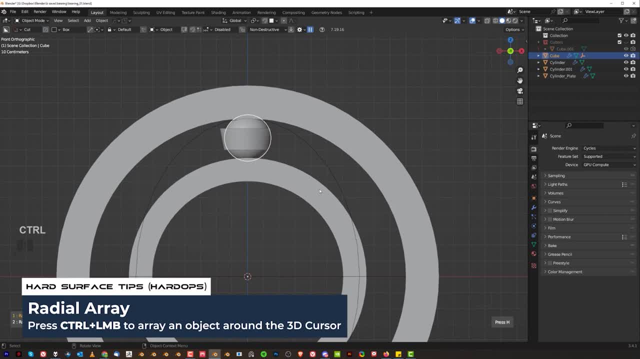 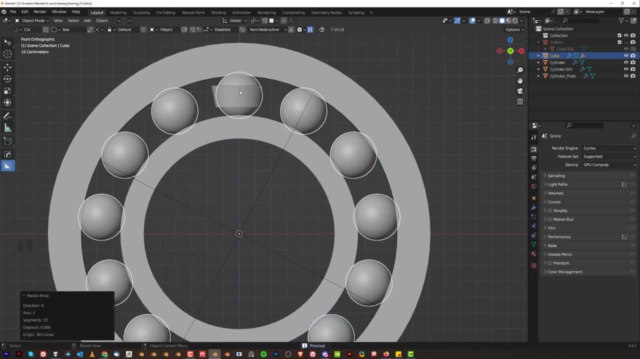 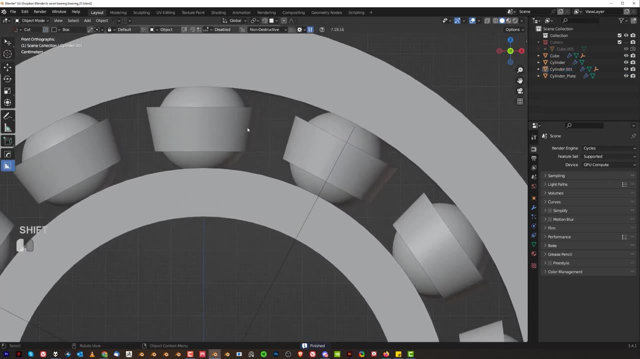 a bearing and we're gonna go to mesh tools and control, click on radial array with hard office X, uh, to flip it, and we're gonna create, well, that many bearings and we're gonna grab the same radio with this one boom. that's done and now we need to create a connection here. 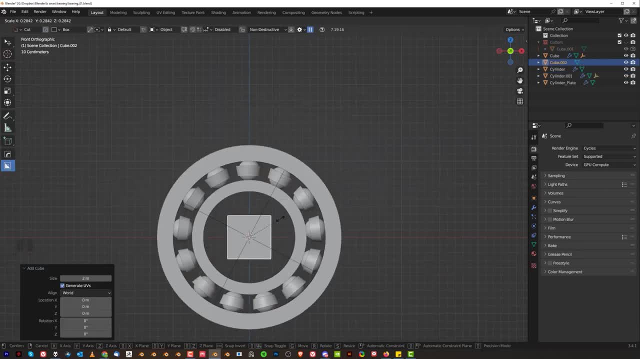 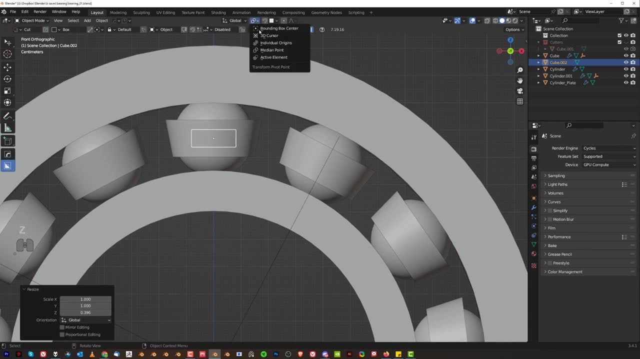 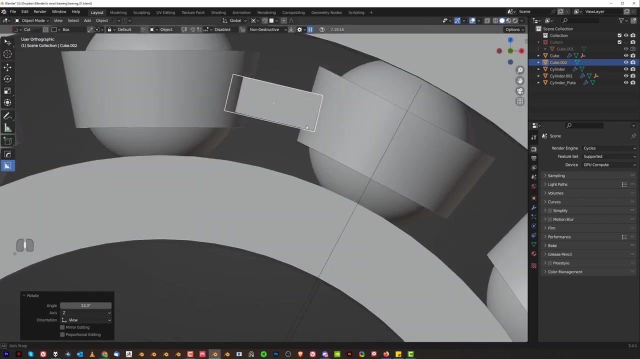 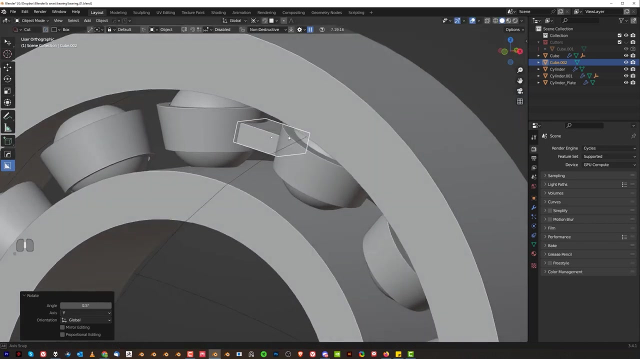 okay. so let's grab a cube and let's go here, jay-z, move it up, scale it and we're going to rotate it on the cursor, so r and just rotate it like this. okay here, and let's just rotate it on y axis. there we go, okay, and I think this will do. 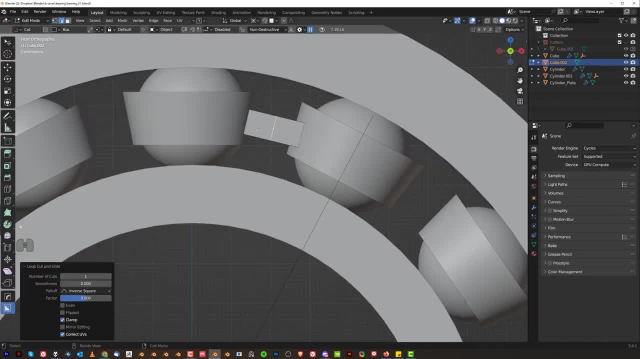 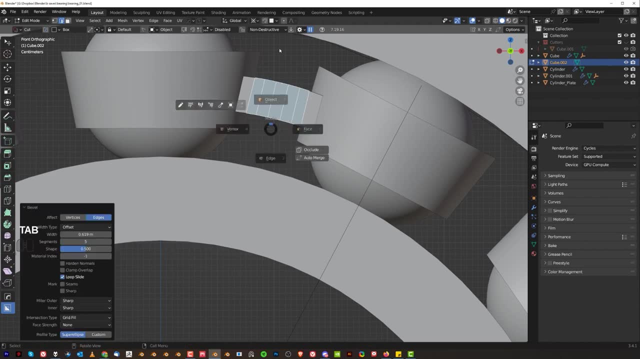 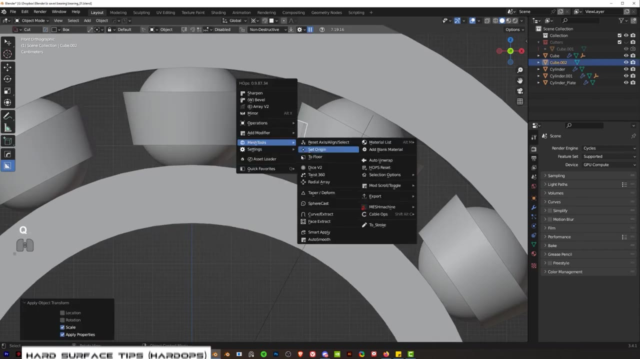 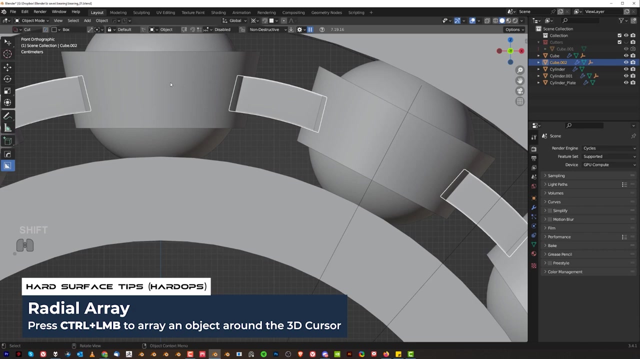 if you really want to, you know, you could uh, um, we could just uh, sort of bevel it a little bit like that right a little bit, so it kind of follows this curvature here, and then let's apply scale and we're going to, you know, array this as well and we're going to add some bevel to it, small one and the bevel here. 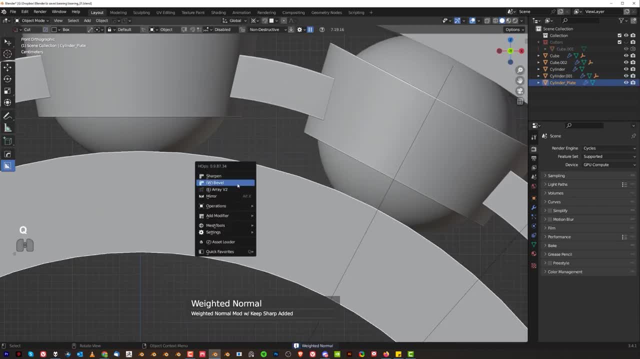 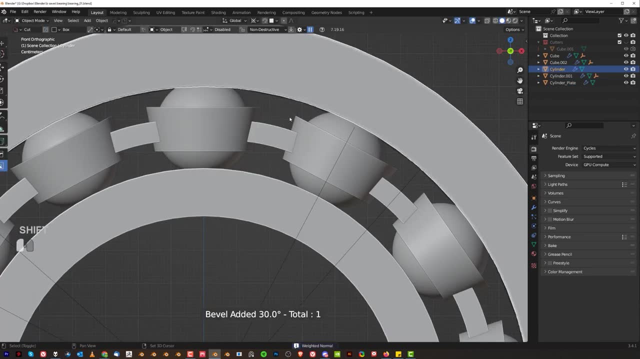 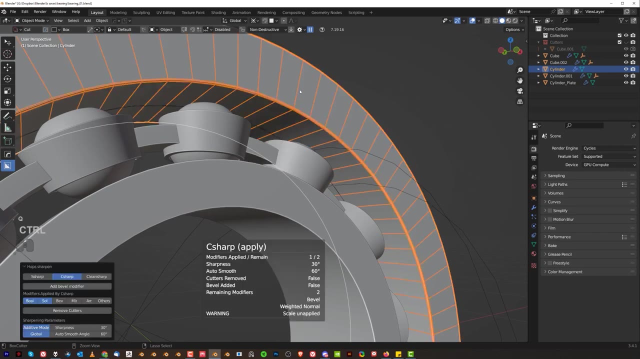 also small one. remember, these are machined parts, so the bevel is going to be really small. yeah, don't make it too big or it's just going to look weak. okay, so small bevel will do it, right, cool. probably this one is still too large, but it's okay, awesome. so now we can apply that. so show up. 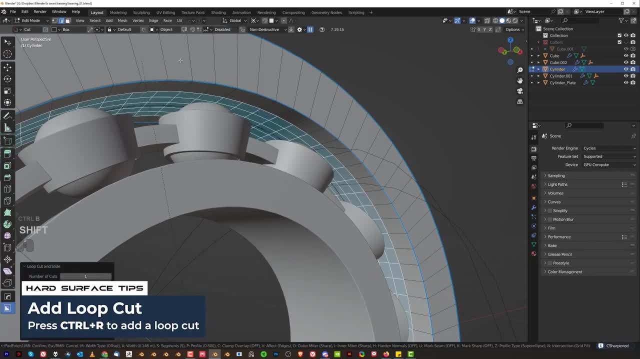 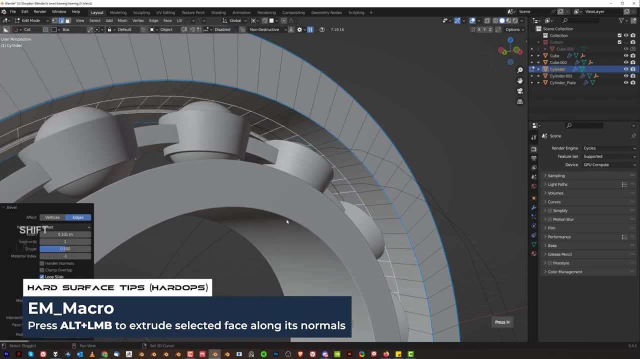 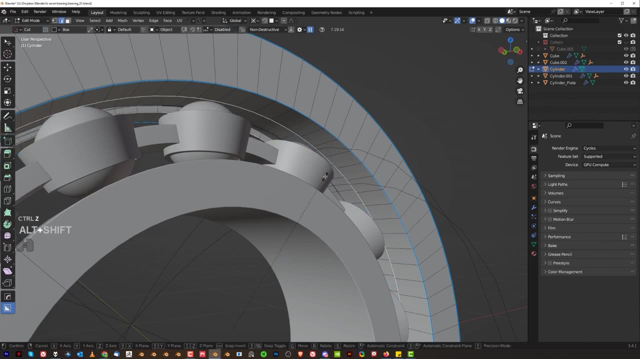 and we're gonna grab the um edge here, split it. so ctrl b and we're gonna create a groove. so q and alt m macro inside, okay, select this, select this edge here and this one and s y, we're going to scale them out and we're going to do the same thing here. so 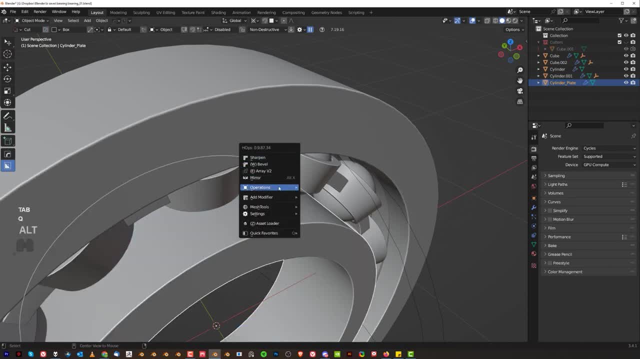 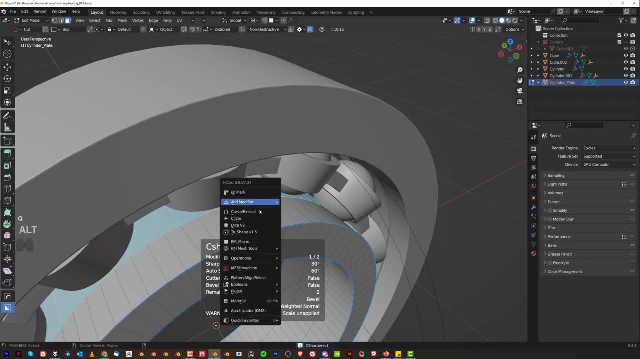 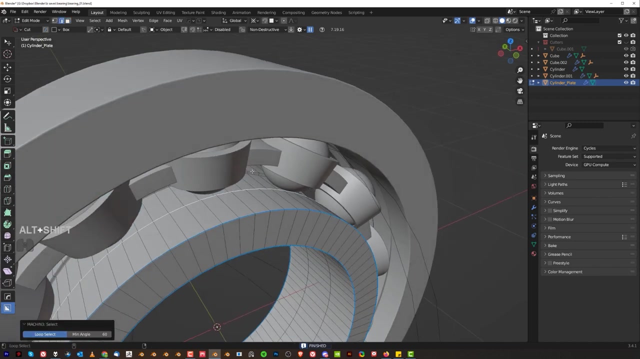 let's just create a groove and alt m macro, alt m macro- oh, we need to apply this. so sharpen and then select this and, um, alt m macro. down there we go, select these two edges and kind of you know, kind of scale them like this and they should do this one. it's a little. 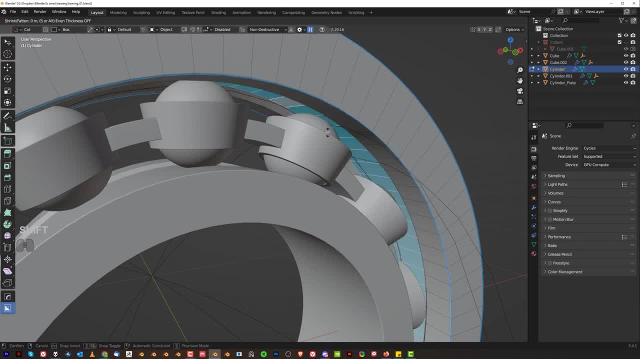 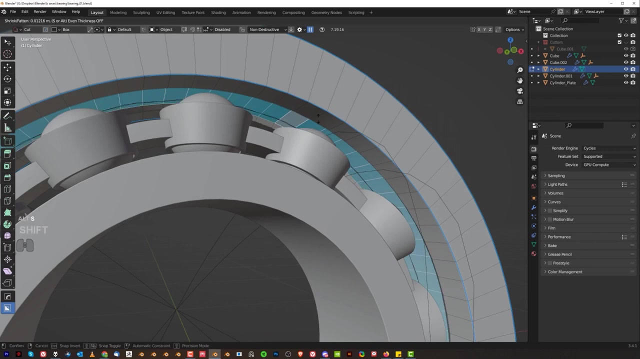 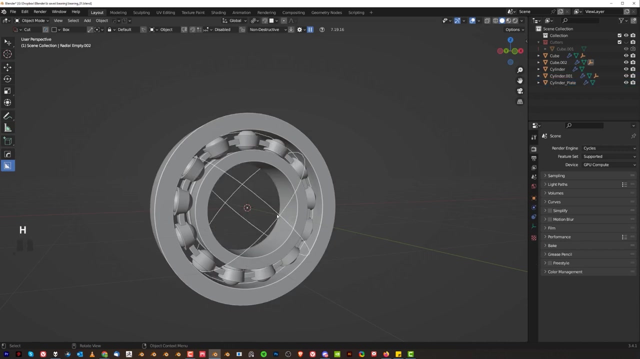 bit too tall, so we're going to bring it a little bit down. so alt s and the, can you know, bring this a little bit closer here. oh, there you go. in fact, we're going to switch this to individual origins and then alt s, that's better. okay, cool. so this is our basic bearing, and now what we need is, um, some kind of 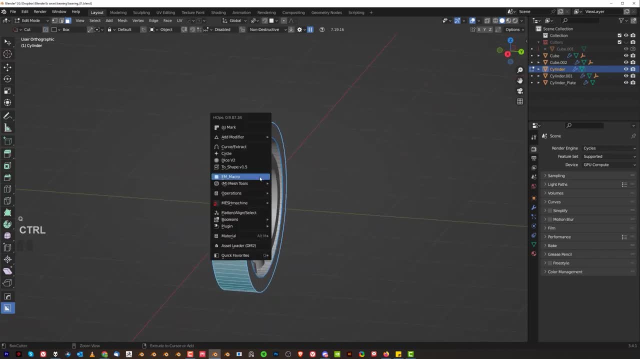 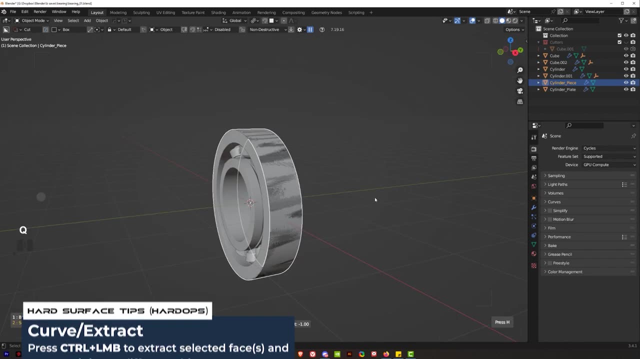 a casing here. so we're gonna borrow this one and, uh, control, click on curve extract to extract this, and we're going to um add a solidification on top of it, maybe a thicker one like this, and move it a little bit to the front. to the front. 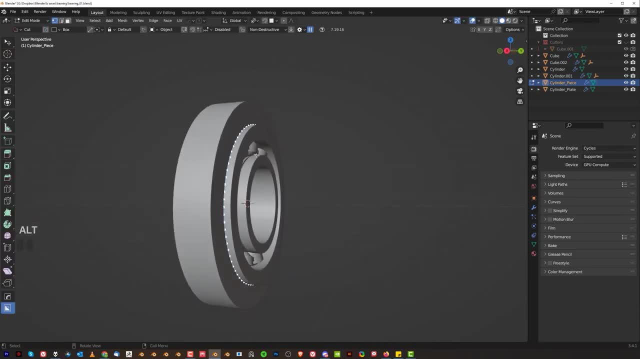 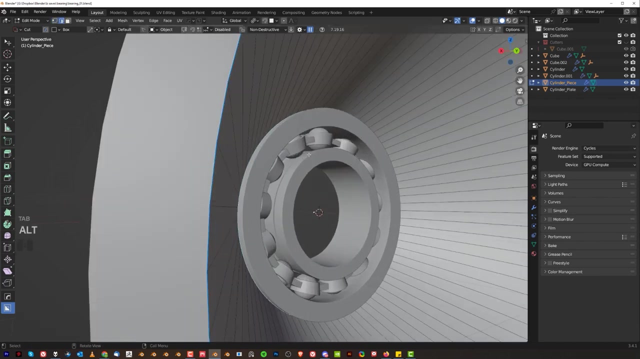 like that, and i'm going to grab this edge here with alt, right, i'm going to extrude it backwards here, okay, and we're going to scale it like this, actually a little bit more, and then scale it like that, okay, cool, and this one could be a little bit deeper. so, gy, and move it a little bit deeper, okay. 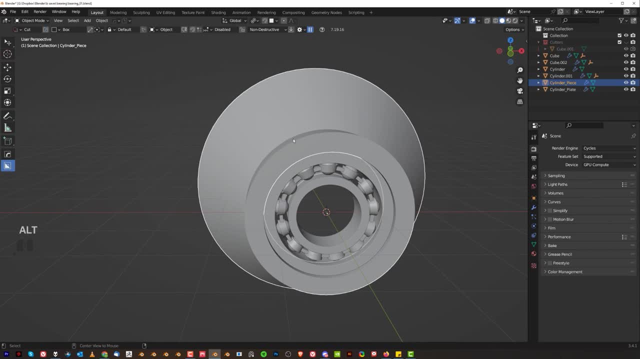 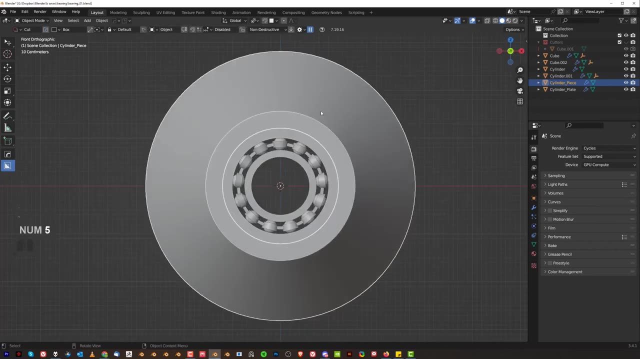 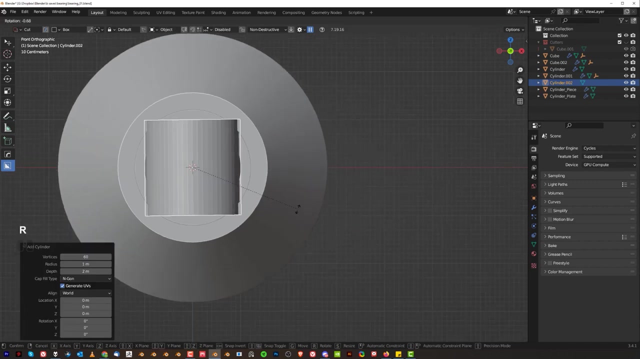 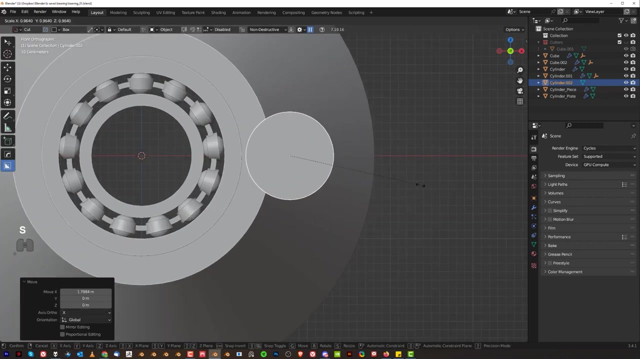 something like that cool, that's, uh, that's pretty cool. and, um, now we can have some fun. so, uh, let's uh grab another cylinder and we're gonna create 60 hertz and our x90, scale it and move it here, scale it a bit more and move it in here. make sure it doesn't overlap here- and we're going to grab. 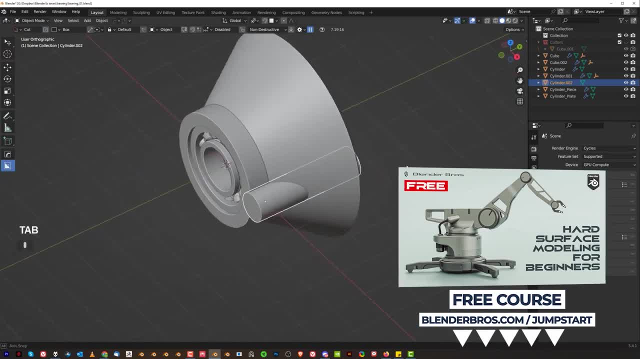 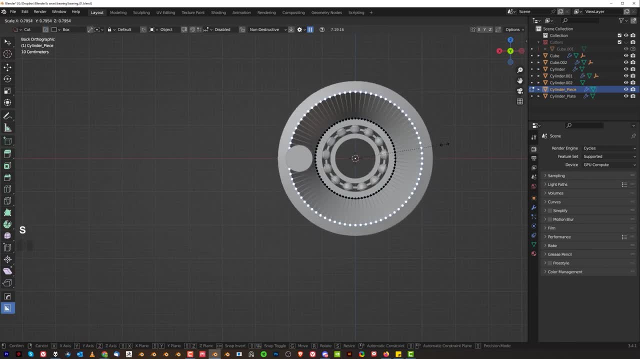 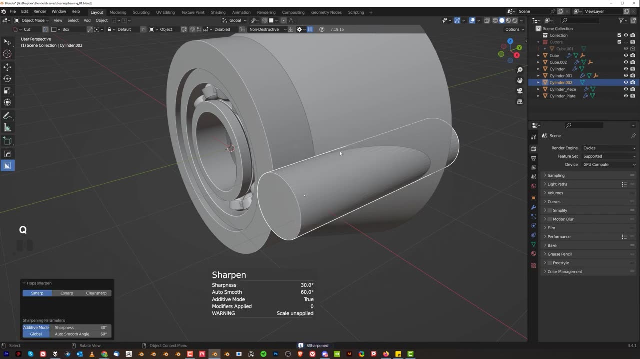 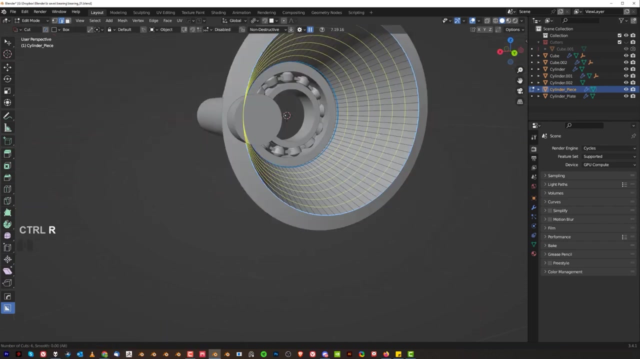 that GY move to the back. cool. this one might be a little bit too too wide, so we can scale it down a little bit, kind of like this: okay, cool, and let's just sharpen this. also need some loops, because we're gonna be merging these, so same here we. 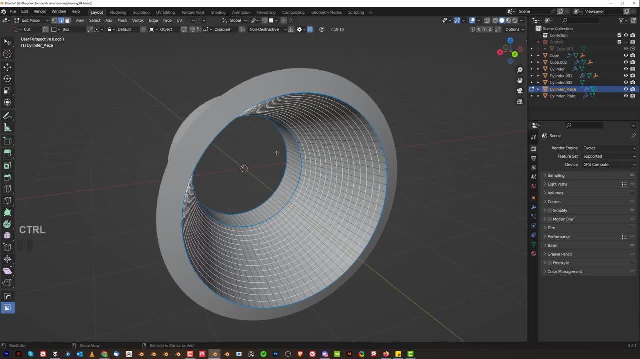 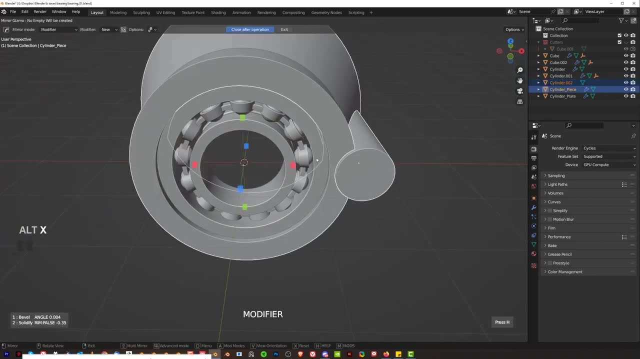 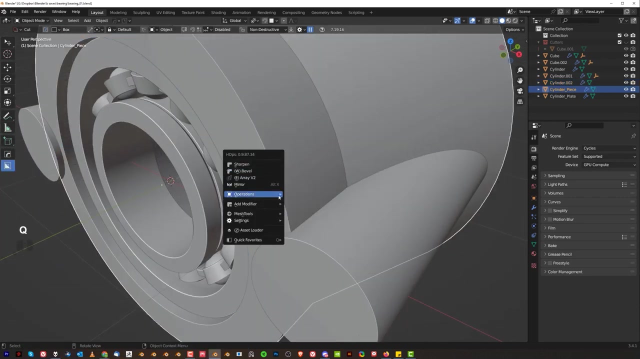 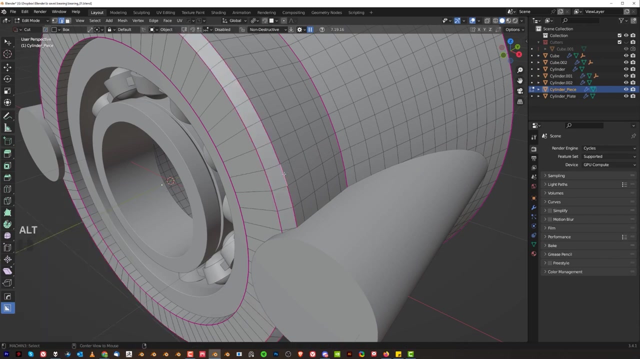 need loops and we also need loops here. okay, cool, so there we go, and we can marry this to the other side. okay, right, so now you're ready to well, kind of ready- to apply this over here. I'm gonna multiply this click, halt, click with mesh machine going to create the chamfer and bevels. okay, cuz you wanna. 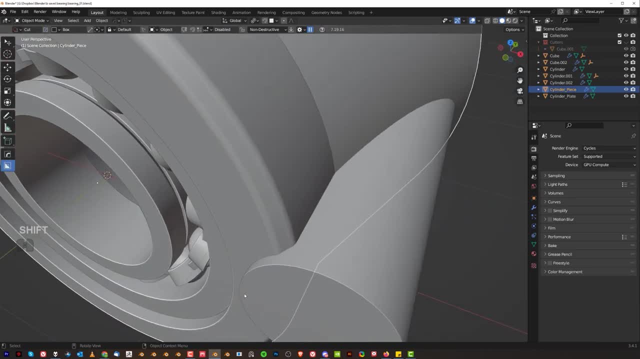 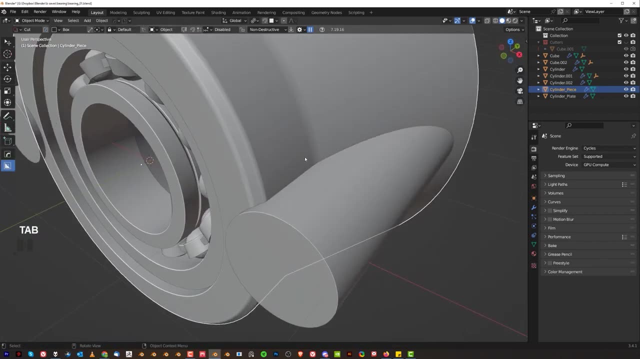 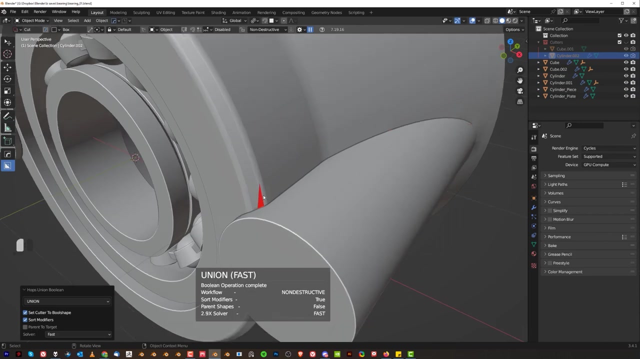 smooth it out. the reason why we're gonna smooth it out? because we going to be running a bevel here, so here too, a bevel, okay, like this peachy, and now we can actually apply this. so click here, click here and let's just boolean this together as a union gonna have. 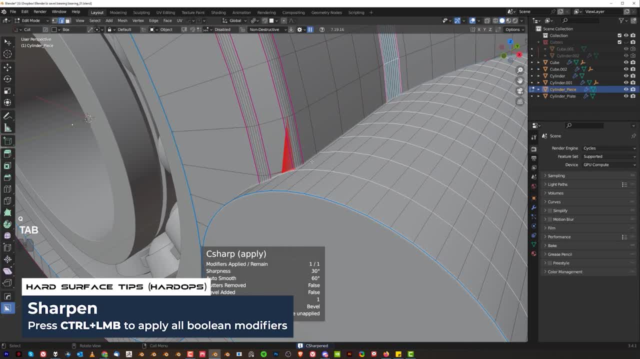 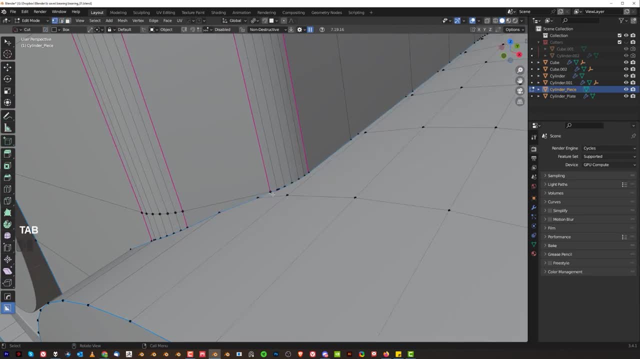 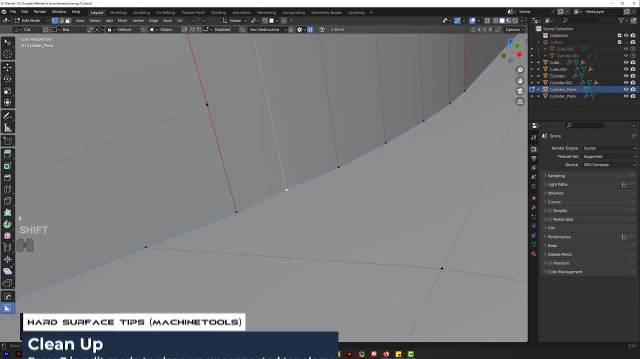 some artifacts here, but that's okay, let's just sharpen this and then let's just turn off the bevel for a second and let me see that this one could be going a little bit higher here, so we could combine these. there's three to clean that. you can remove this one and this one should. 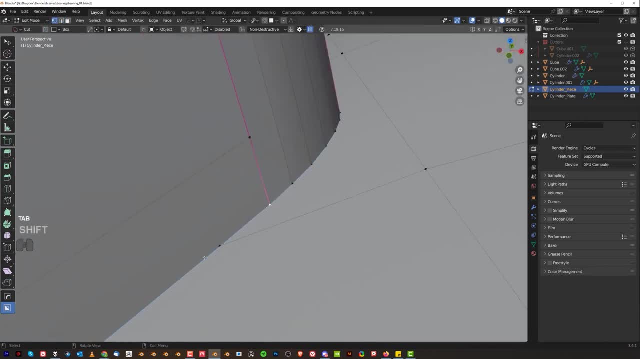 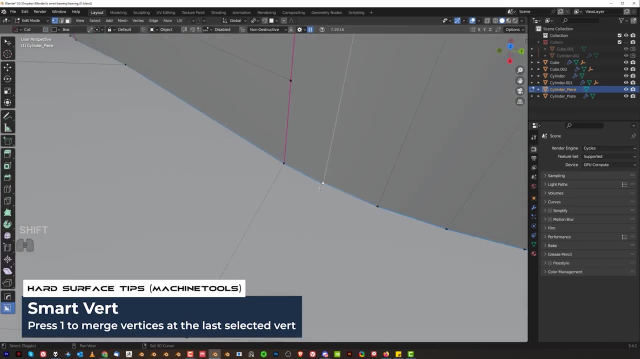 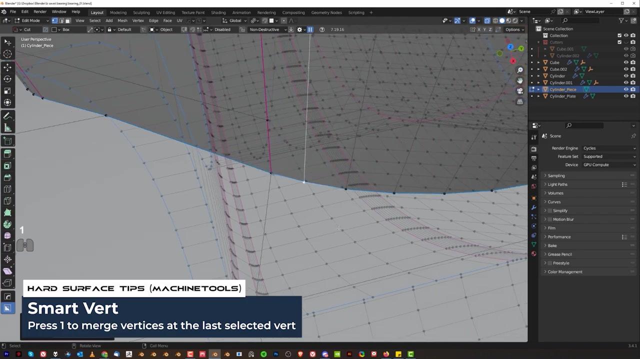 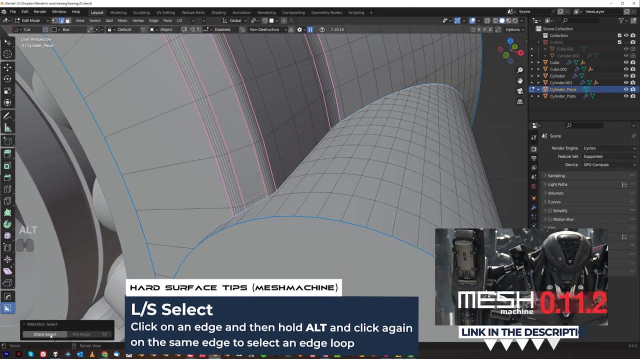 be a sharp edge. what the hell is going on here? you know, let's combine these and there is some problem in here. let me go to occlude. you see that. ah, there we go. press three on the time. they should do it, okay, all the time. click out, click and. 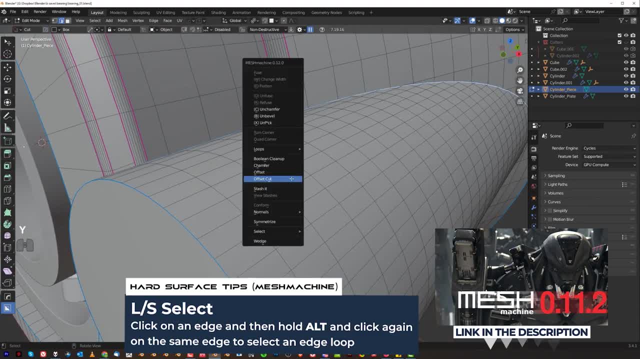 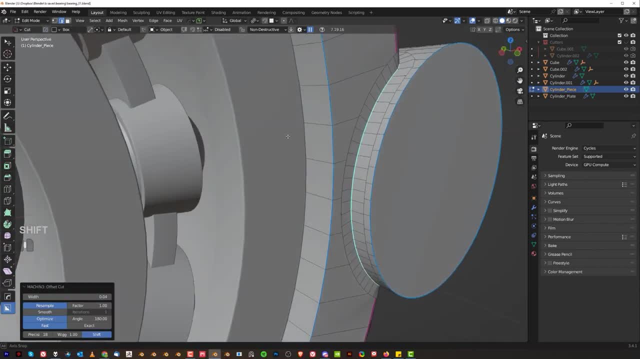 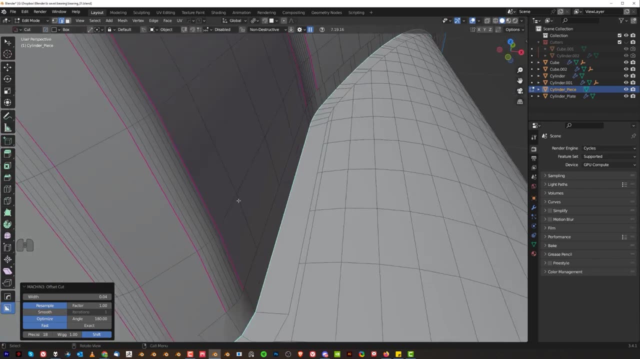 select and y and offset, cut. now we're talking. now we need to choose the correct amount of this, the factor. i think it's okay we could smooth it out, so it's going to be a bit better on the curve, but actually in our case maybe not. we do need some more resolution here. so let's just add that. 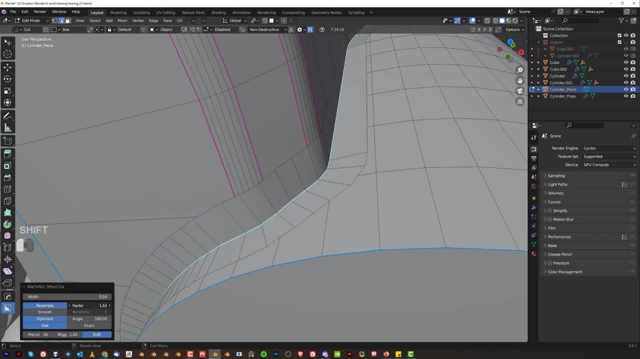 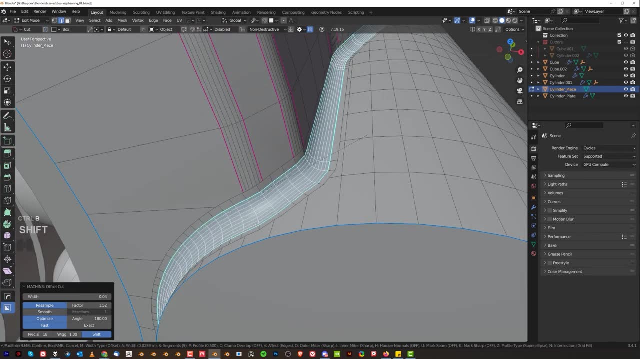 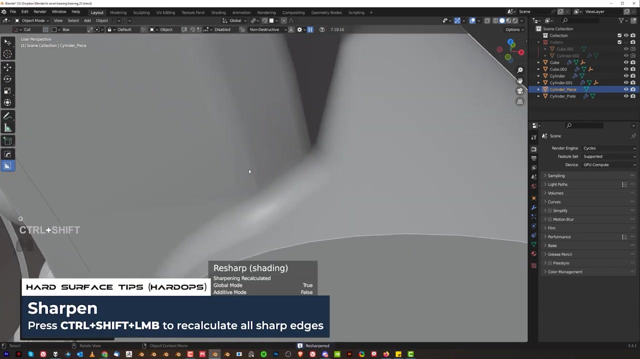 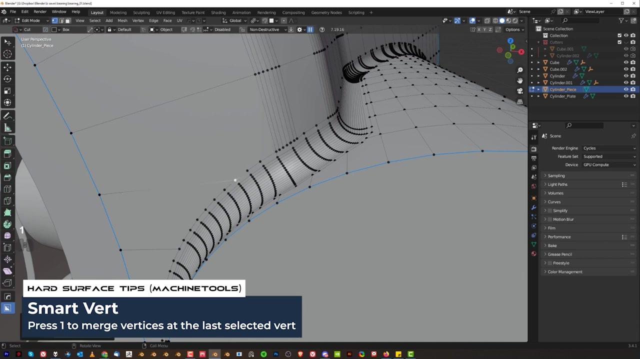 here a little bit more s on this corner, nothing gets better. and we're gonna run a bevel here, okay. so on the bevel here and that's that, and then we're going to recalculate shops and then we need to clean it. so, uh, here we can combine that and we can combine this. 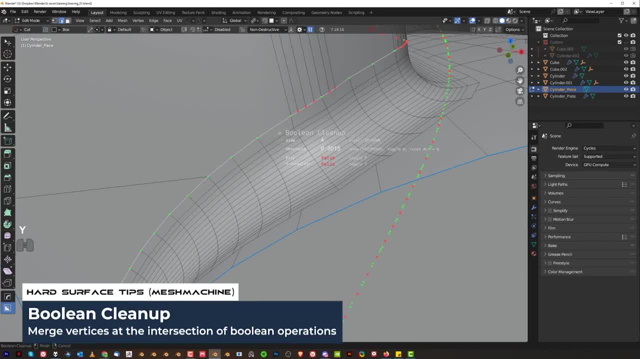 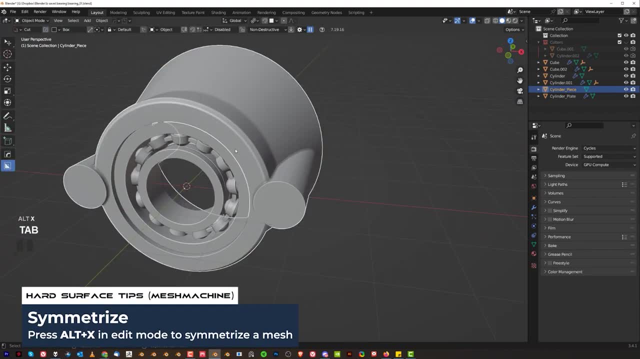 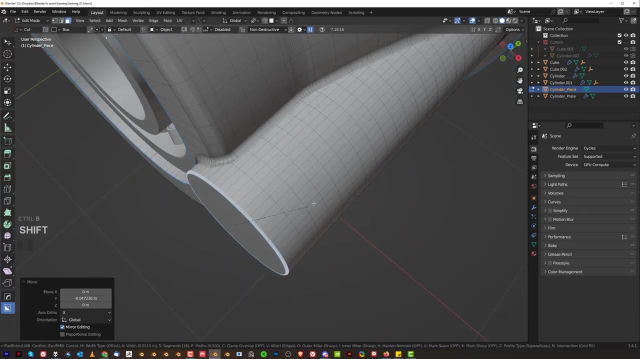 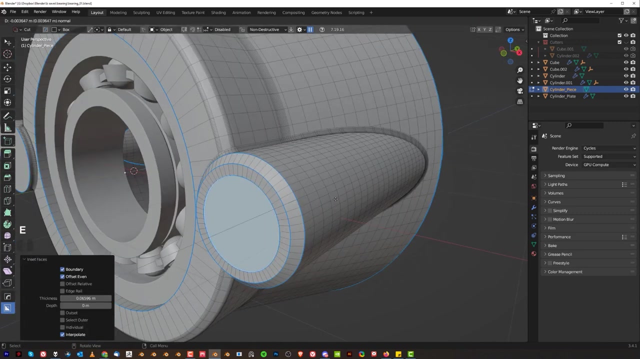 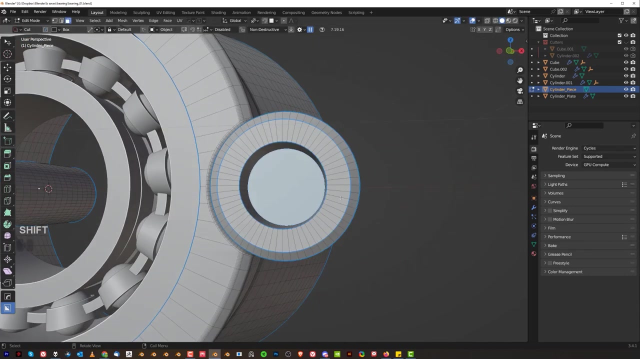 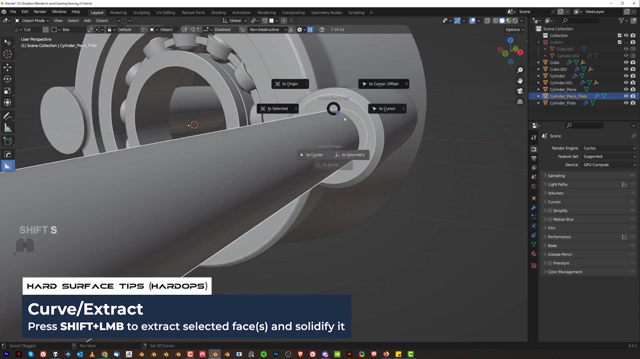 right and click alt click and y and boolean cleanup. scroll your mouse and connect these- the set side, and then we're going to extrude it. actually, let's make it thicker it's and make it longer. scale it in on individual regions. so shift s into geometry. scale it in. 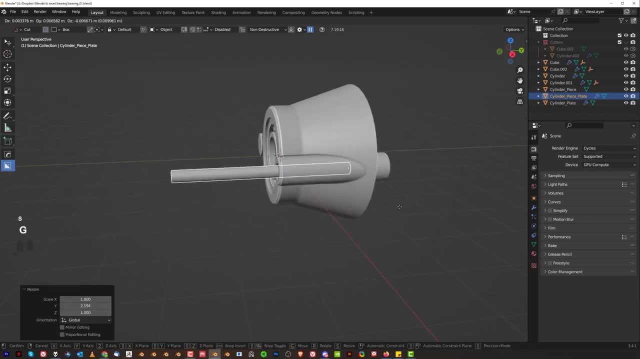 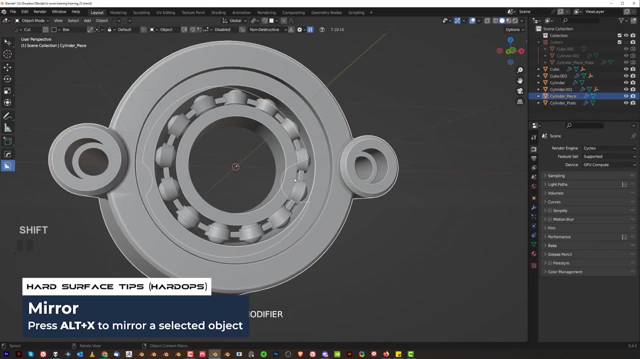 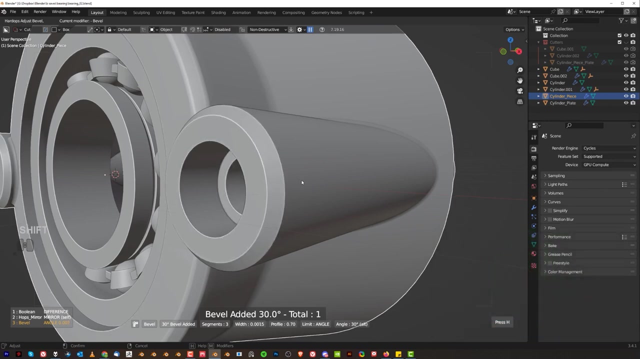 move it across and just let's make it longer and basically difference right, so we got that. and move to the other side. let's just save it because reasons and now kind of the battle. okay, so small one guys, small, this is a machined piece. you need this mobile here we're gonna. 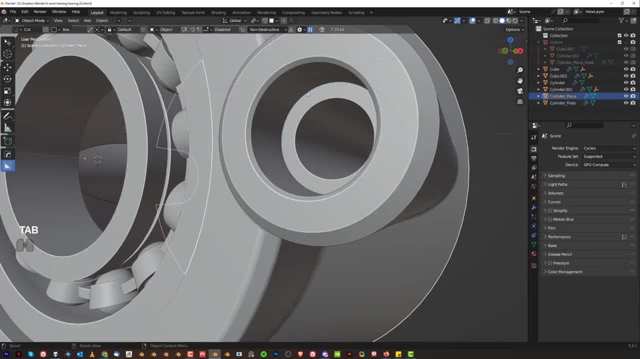 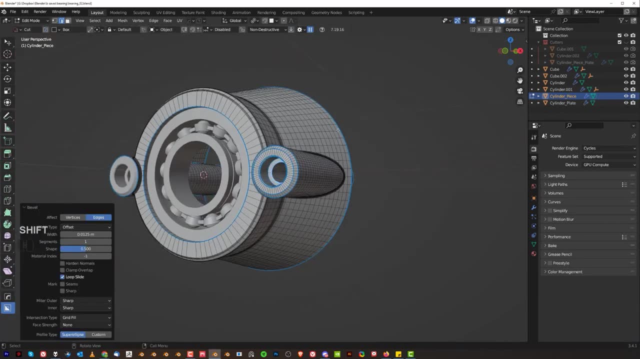 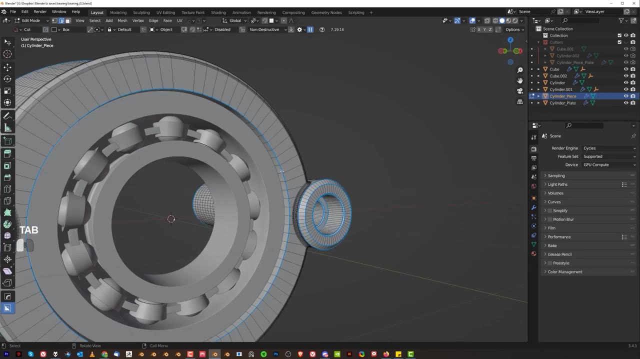 have a chapter, but smaller one, okay, and we also can have a job over here. so sharpen that and click, autre, click and you know. so much effort here. okay, cool, and now I'll text here inside. that looks really cool, awesome. here too, we give some Chamfались to click out, click and you. 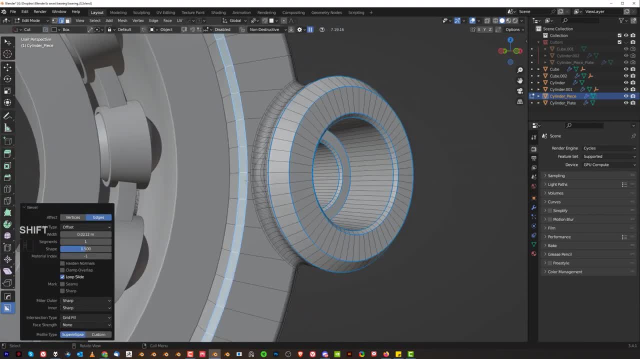 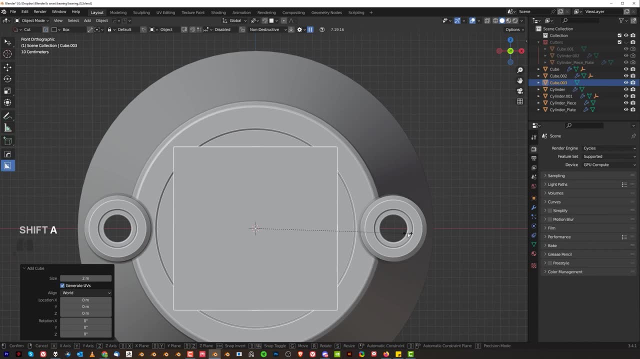 know, at a little bit of a chair, for I don't over do it, because if you do, you gonna have an overshoot here now. so lol, lol, lol, lol. on this piece we could have some cuts, so we could grab a cube and scale it and move it up here and 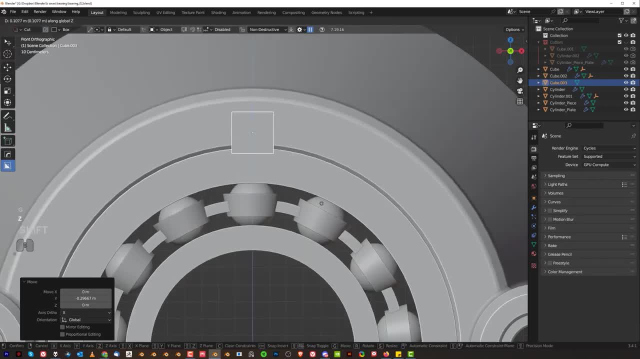 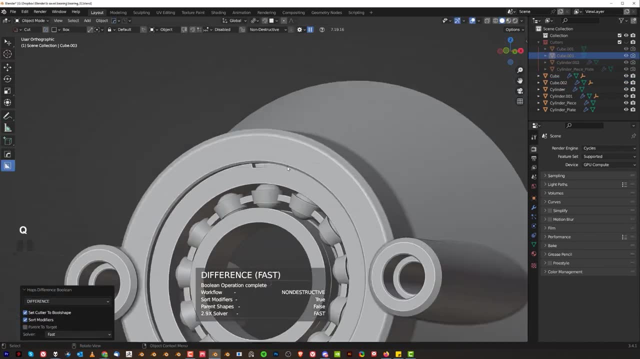 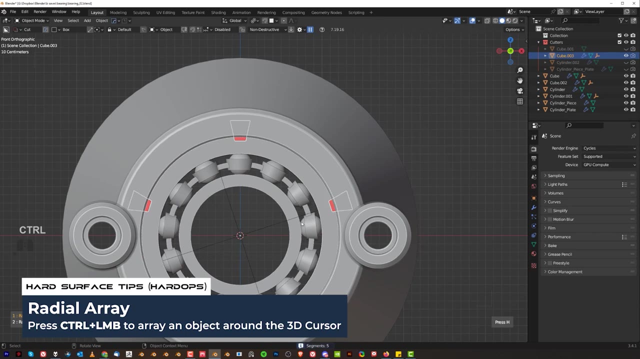 move to the front and just cut it in here, but before we do sx and scale it, clear keystone effect and difference. and then we're going to recover this and q and control. click on radial and let's create maybe five. it's now so it's gonna offset a little bit nicer here. top. 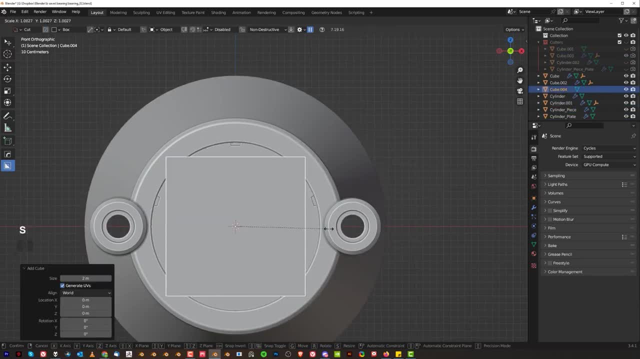 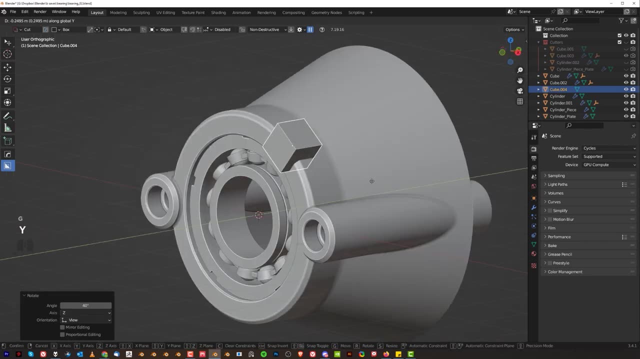 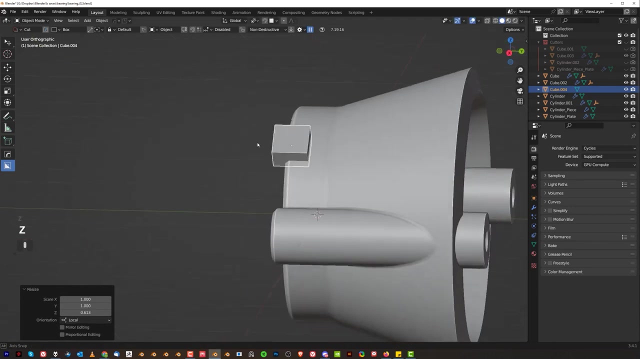 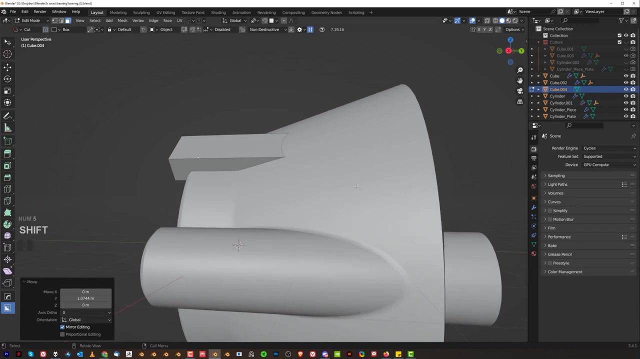 we have some brackets, so maybe another cube and scale it, move it to the top switch to cursor, rotate it, holding control, move it forward, all right, and let's scz on individual origins, okay, move it backwards. sync it in here. it's gonna look pretty cool. actually, maybe not. maybe let's do this. 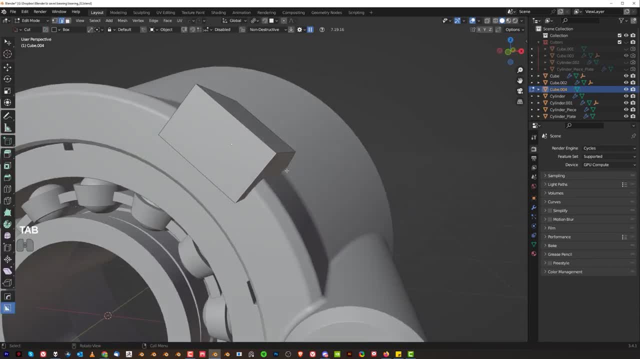 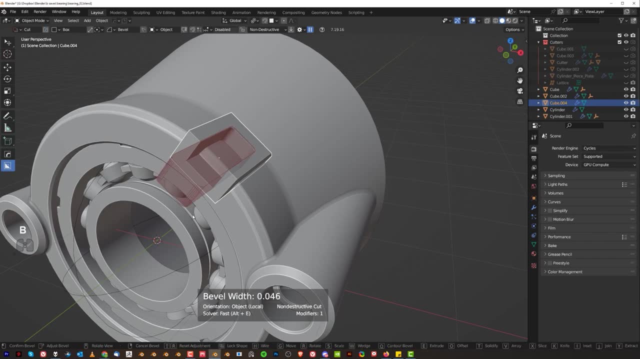 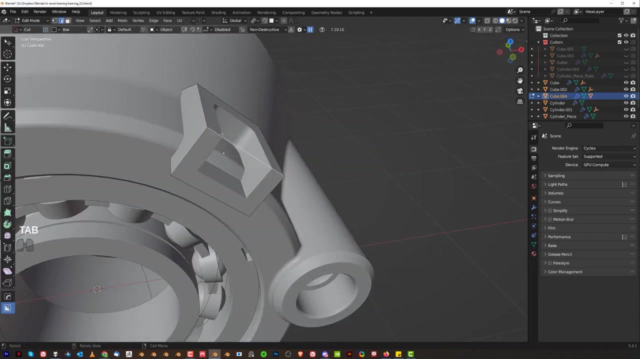 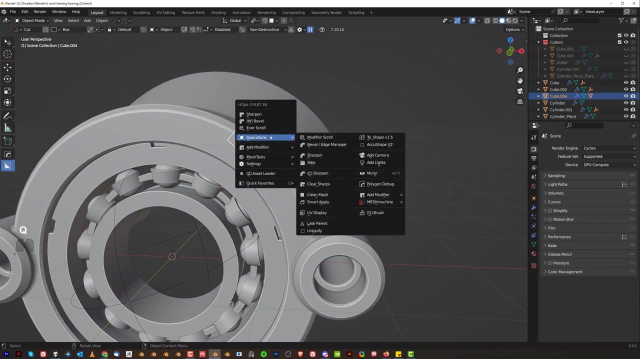 well, that's interesting and here we could have, um, you know some, some cuts like that. okay, let's just mirror this to the other side and, uh, you know, this could be actually, this could be chamfered or beveled or whatever, and we could. let's apply this so operations multiply, shift, click here and hold shift and mirror to all sides. 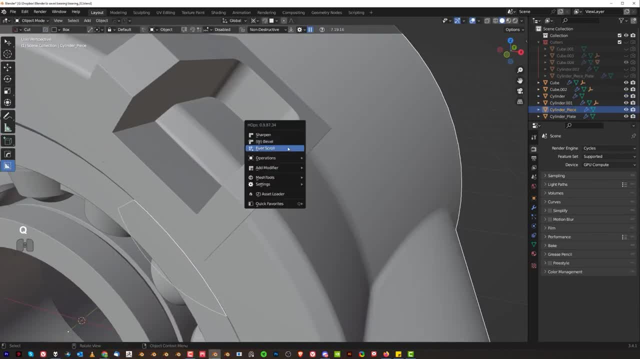 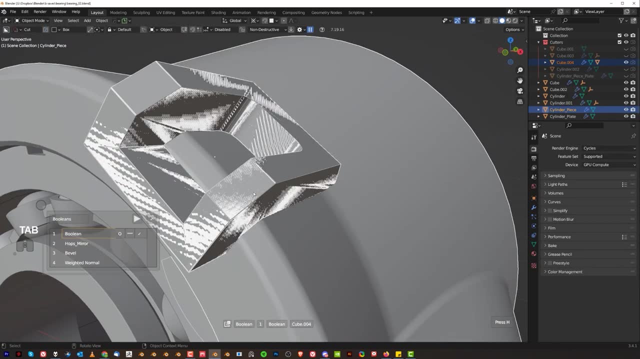 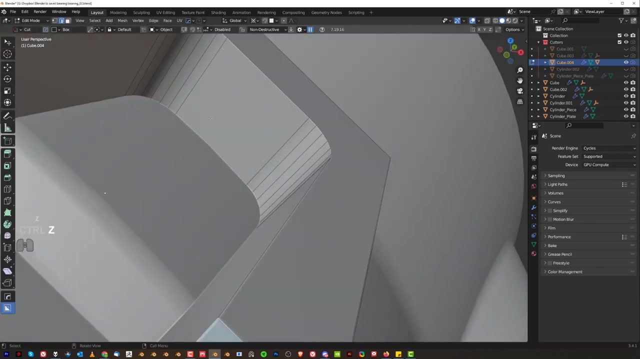 so you're gonna get this bracket. let's run some loops here on this cutter, so i need some drink. my throat is hang on, that's better. i'm suffering from some serious pollen um allergies. it's bloody terrible. but what are you gonna do? right, hang on, hang on, hang on, this is um here and then. 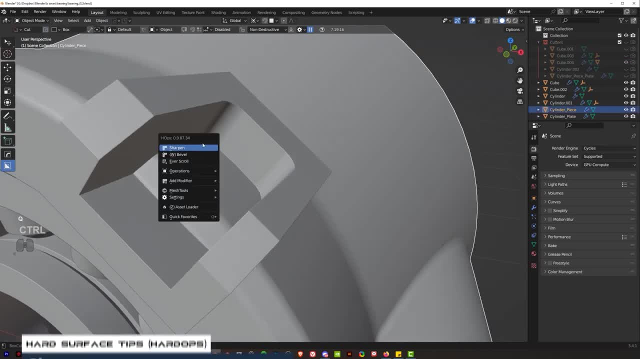 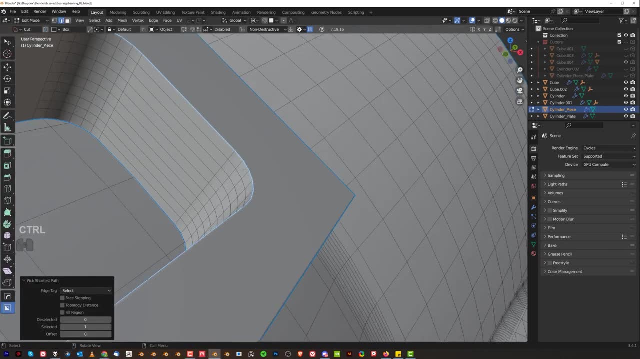 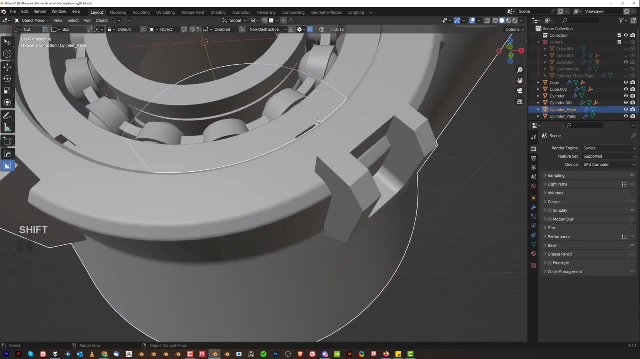 let's do that and i think it's gonna be fine. so now here, sharpen, there we go, and we can run a jaffer here on this, just don't overdo it. there we go, and this should mirror to all sides, if it doesn't, uh, simply, you know, run. 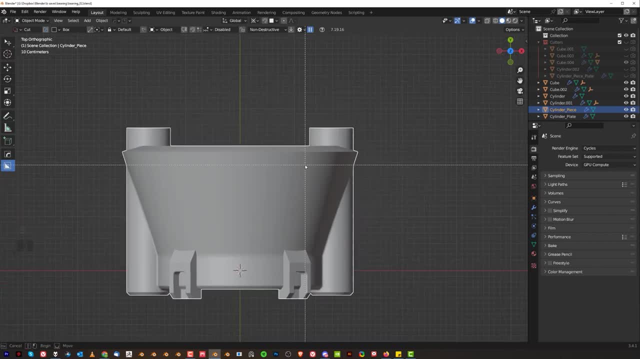 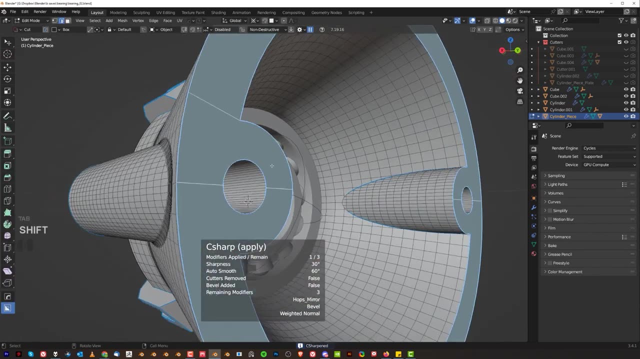 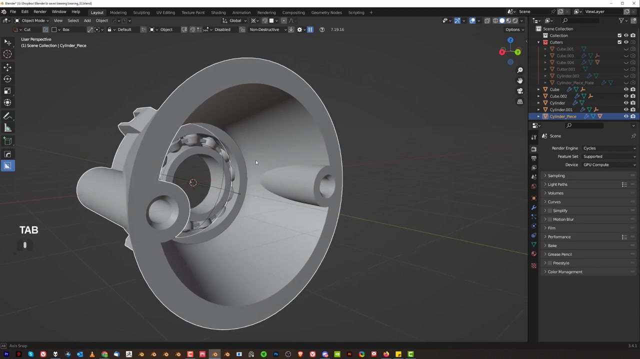 a mirror with machine tools and here what we can do so you can slice this like that and the backs is going to be nice and uniform. also kind of flush here could have some you know chamfer here, alt x and you know you're good to go. 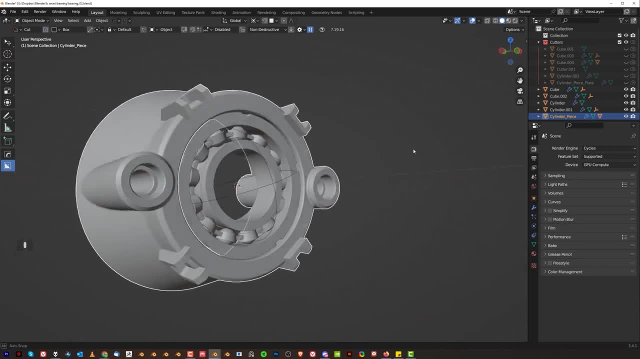 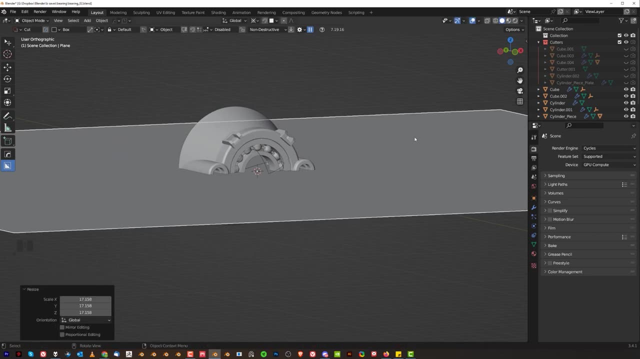 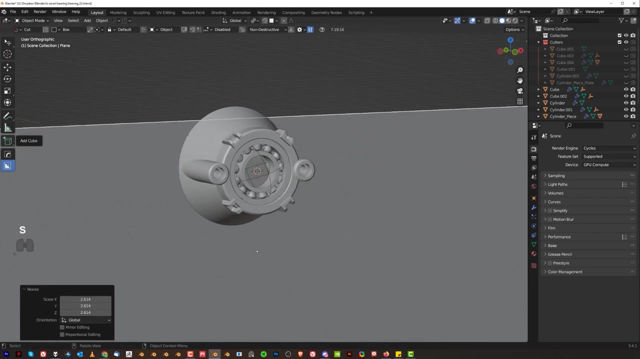 that looks pretty awesome, cool, cool. and that's our final piece. so now i'm gonna, you know, texture this very quickly with our blender bros mods. i'm gonna show you some new mods we've created recently. um, they're still in development as of recording this video, but if you're watching this, 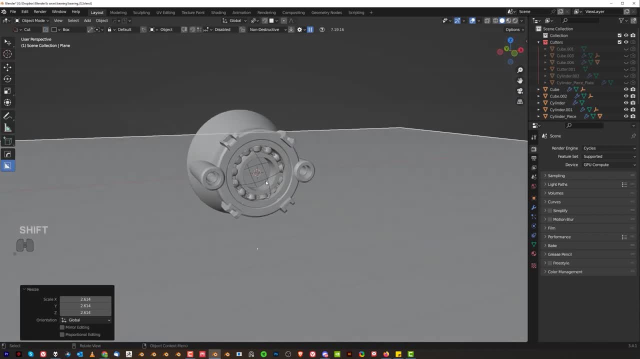 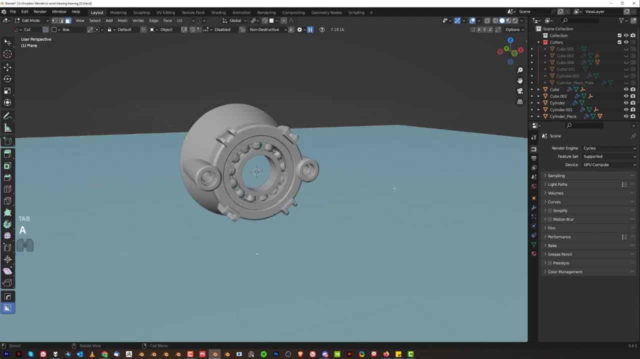 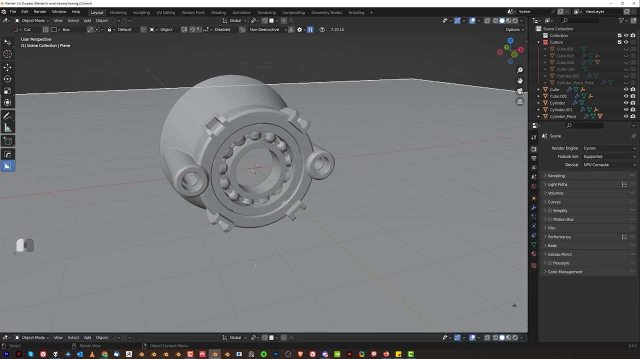 in june, july, you know, maybe the pack is already out. so go ahead and, you know, check it out on our website or possibly on blender market- we haven't decided yet, definitely not gumroad, but, uh, you know, blenderblastcom or blendermarketstore anyway. so let's go to um here to not to shader, to assets and 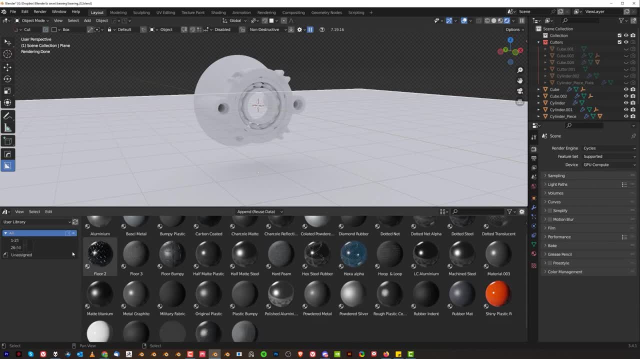 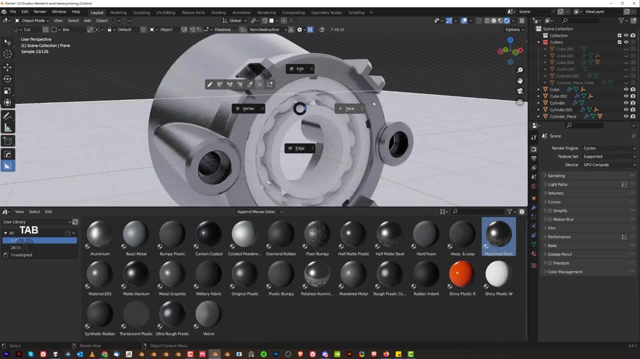 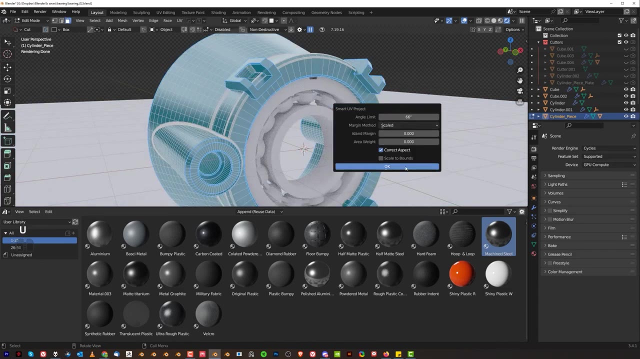 render view cool, and i'm going to be using, uh, these mods here so we could grab the machine steel, which is really cool. now, um, you're gonna have to unwrap this once the item drops, but, um, i still have to unwrap this mesh here. so you and smart tv project, and here too, in smart tv project. 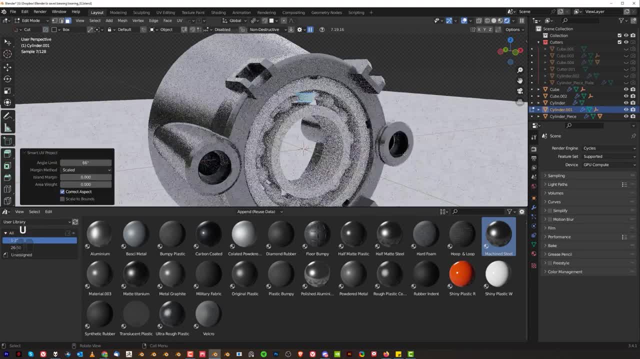 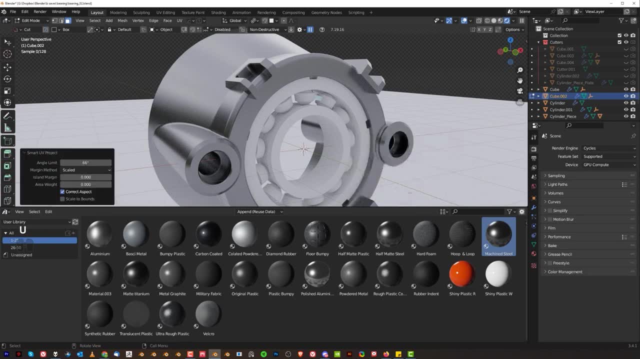 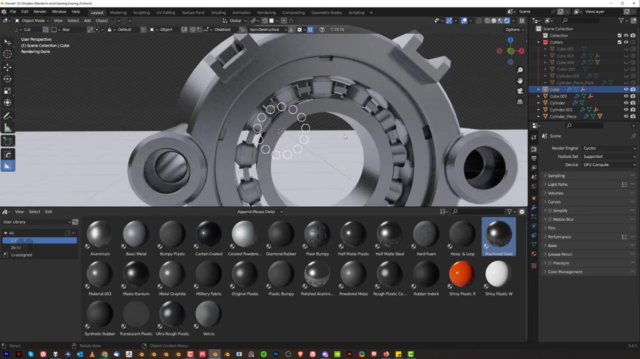 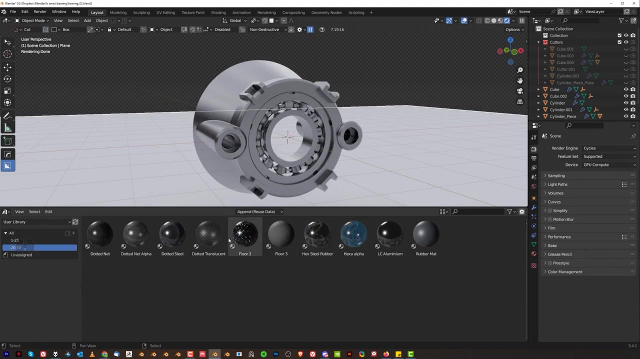 and smart tv project, and here too the small one as well. and the bearings, well, we can't see them. but you know, just for the health tutorial, let's do it properly. so here we're going to be applying all these, the same mods. really, here it looks pretty good, awesome, and the floor we could have on this one. 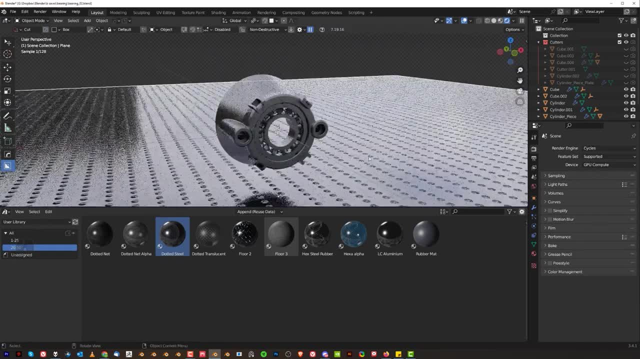 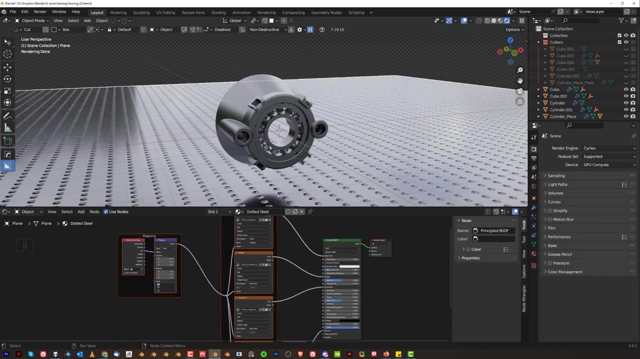 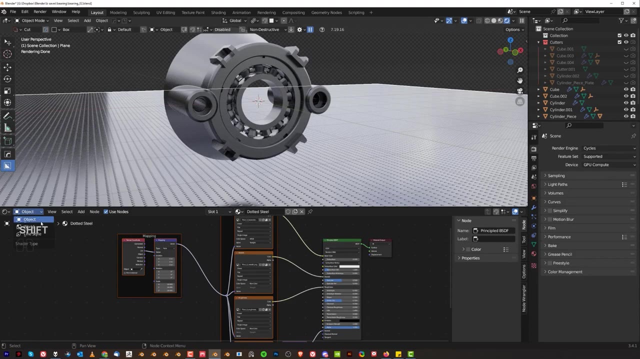 dotted steel, which is pretty awesome. right, cool, we just have to change the scale. uh, so let's go to shader and change the scale to maybe i don't know 10.. there we go. it looks pretty decent. now, of course, different lighting. i mean, we could switch the lighting to um, something else. 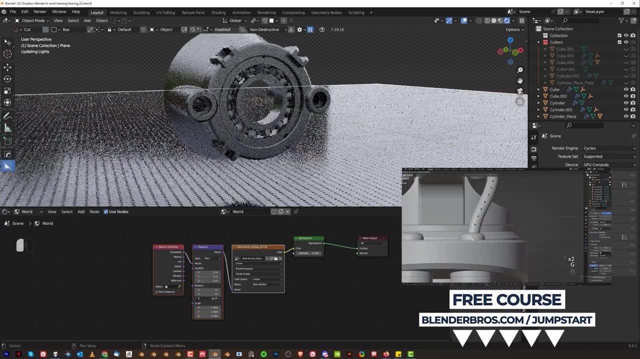 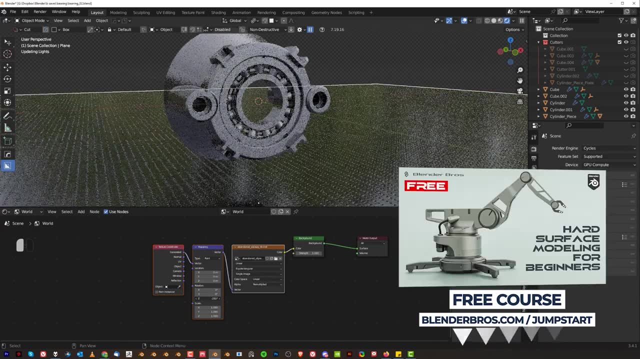 uh, but i'm not gonna be doing it here, i'm just gonna rotate it to make it a little bit, you know, more presentable. so the lighting comes from the right hand side and sort of, you know, highlights this front here up just to 1.8, so it's brighter.